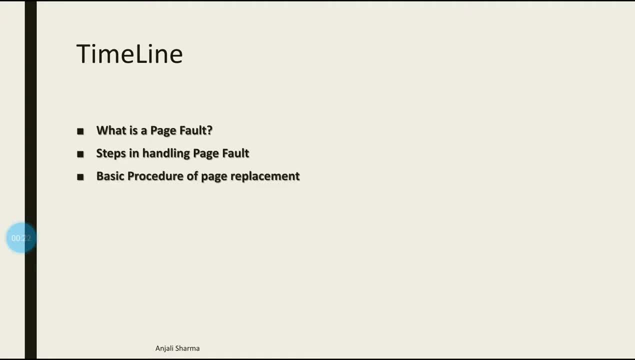 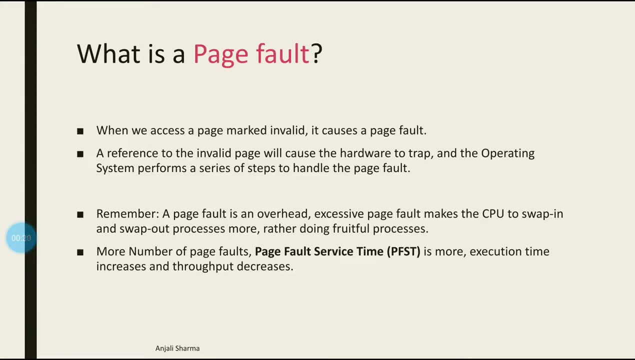 the steps handling in page fault, the basic procedure of page replacement and the concept of modify bit. So what is a page fault? When we access a page marked invalid, it causes a page fault. A reference to the invalid page will cause the hardware to trap and the operating system. 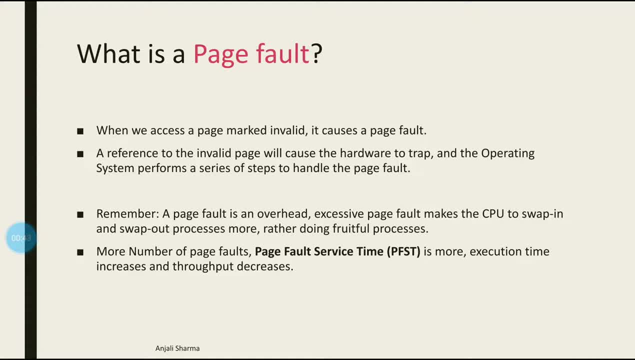 performs a series of steps to handle the page fault. See what happens: whenever we need to access a particular page, we refer to the page table where its corresponding frame number is written. But suppose if our page is a page fault, then we refer to the page table where its corresponding 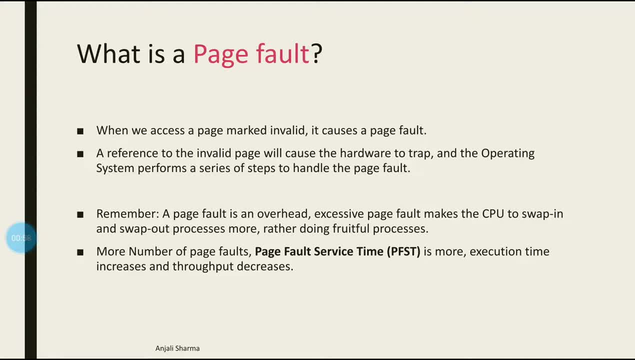 frame number is written. So to identify the page fault, we added an extra bit in the protection mechanism that is known as the valid and the invalid bit. So if we refer to a page whose valid and invalid bit is set invalid, then we call it page fault In general language. 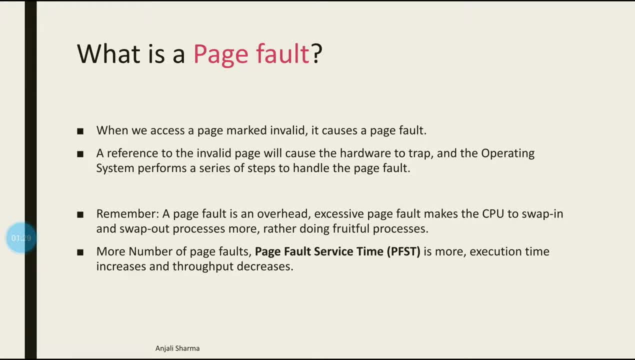 we search for a page, and if we don't find that page in the main memory, then it is a page fault. So in such a situation the operating system is generated a trap and the missing page is fetched from the secondary storage or backing store and brought. 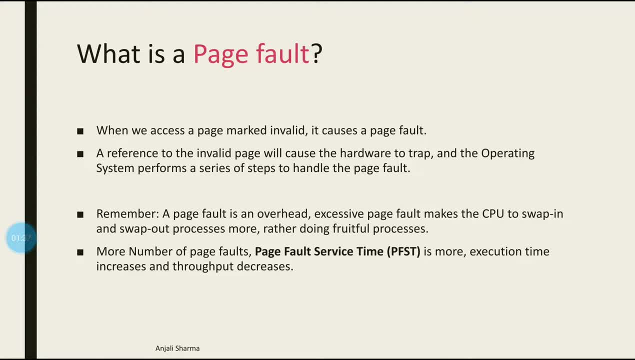 into the main memory. So that is the handling mechanism. Remember that page fault is an overhead. Excessive page fault makes CPU to swap in and swap out processes more, rather doing any fruitful calculation or processing More number of page fault means that the page fault service time. 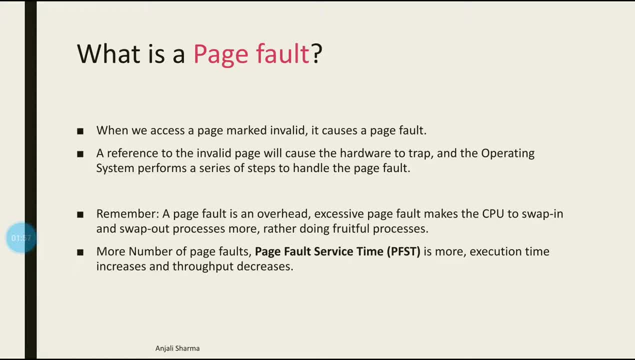 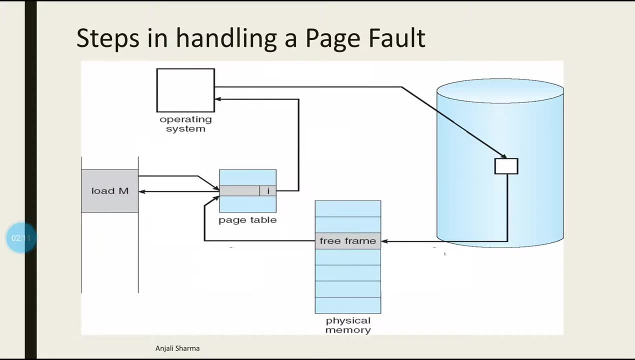 that is, the time taken to handle the page fault is less than the time taken to handle the page fault. Is the page fault, service time is more and the execution time increases. therefore, the throughput of the complete system will decline. So let us see the steps involved in handling the page fault. 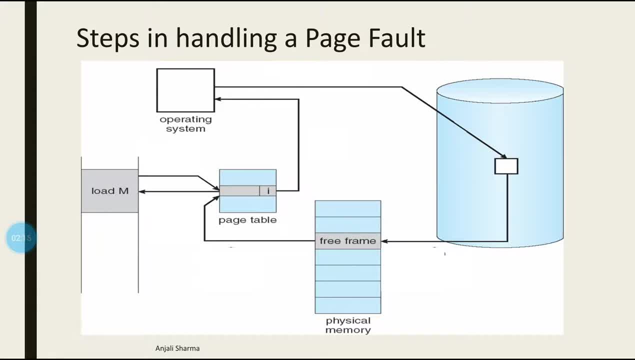 We have a page that is M and the instruction says that we load M to execute it. So the first step will be that we will reference the page table. So when we refer to the page table to know the frame number, then we identify that the bit was set to invalid. 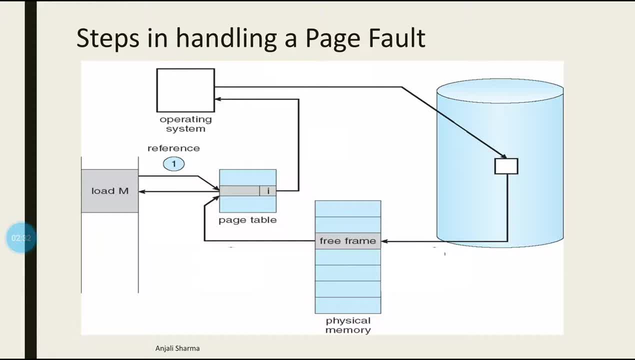 That means we will not get that page in the physical memory. So therefore, a trap will be generated to the operating system, So an error message will be generated to the operating system, which will be used by the operating system to invoke the memory management of its kernel. 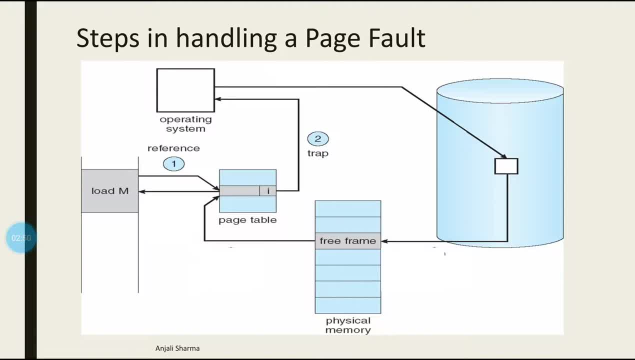 that a page fault has occurred so it has to be handled. So the operating system will find out that particular page in step number 3, in the backing store. So the operating system will find out place of that page M in backing store. 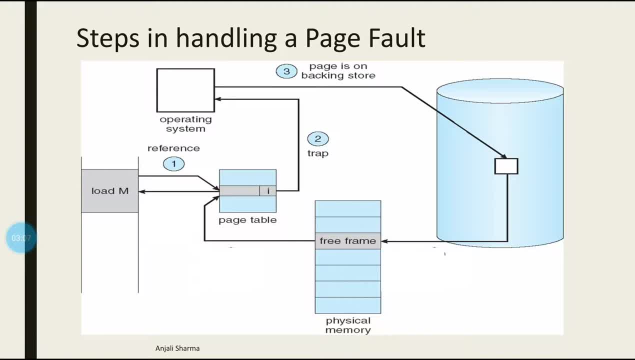 that means in secondary storage in your hard disk, And after identifying that particular page in the backing store, The operating system will bring that missing page into the physical memory. So in step number 4 here, what will be done to the physical memory? 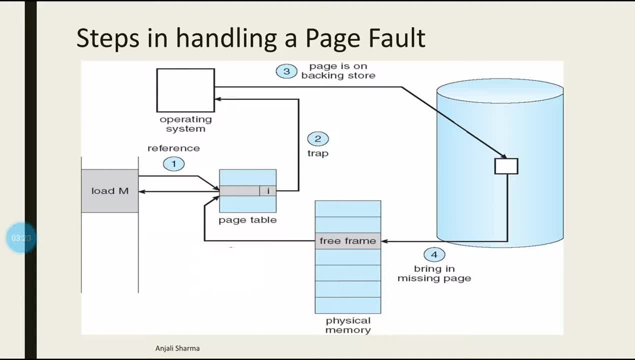 A free frame will be found and through that free frame we will take that page, number M, to that location. that will be left. After that the page table will be reset or modified, because now that page is not invalid. Now it is in the main memory, in the physical memory, so it is a valid page. 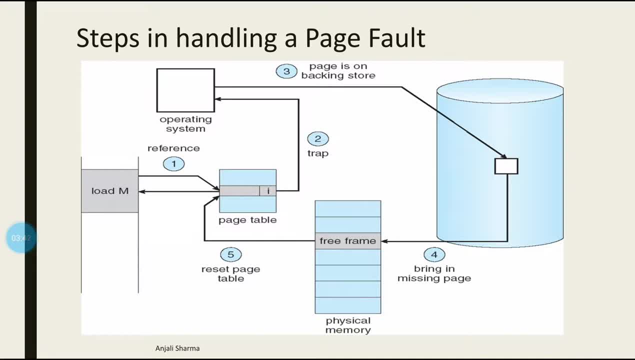 So where the i is written, it will be made valid from invalid And again we can restart our instruction in the last step. So these were the steps that were involved in the handling of your page fault. Now the most important university question is: what do you understand by page fault? 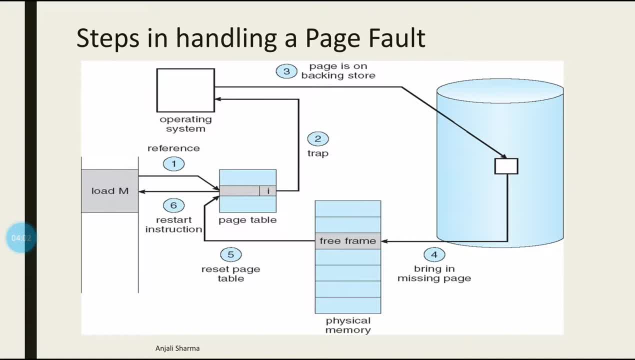 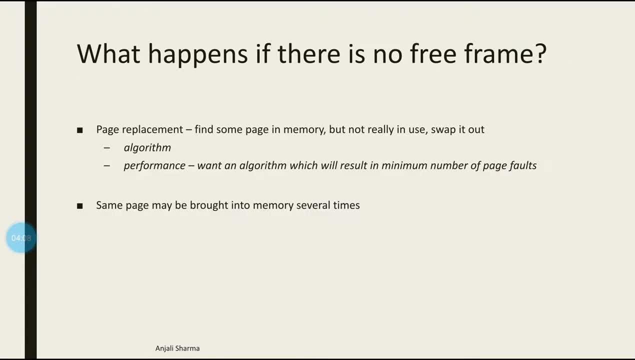 And also write down the steps that are involved in handling the page fault. So if you want these written steps, then you can refer my lecture notes. Now the next thing: what it is that operating system? we just saw what it does is it brings the missing page from the backing store and stores it in the free frame. 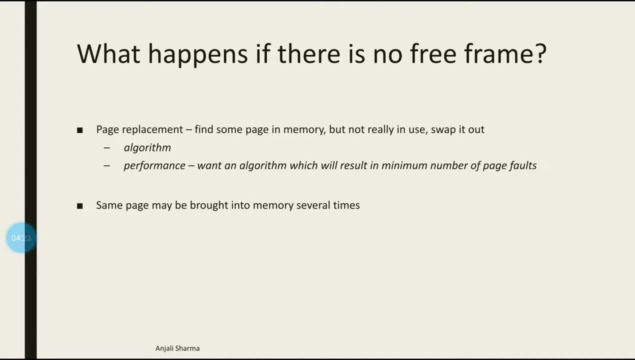 So what happens if there is no free frame, Right? So in that particular scenario, if we tried to load the pages from the backing store in the physical memory and we did not get any free frame, then what will we do? So in that particular situation, we have to do page replacement. 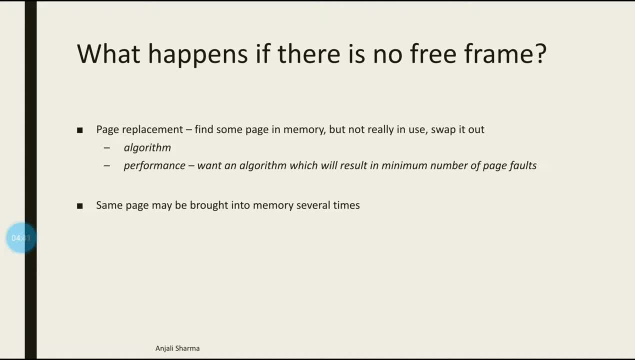 That means our physical memory is full, so we will remove some pages from there and keep them in the backing store. Now, which page should we remove from the memory and keep in the backing store? We had seen this example in demand paging as well. 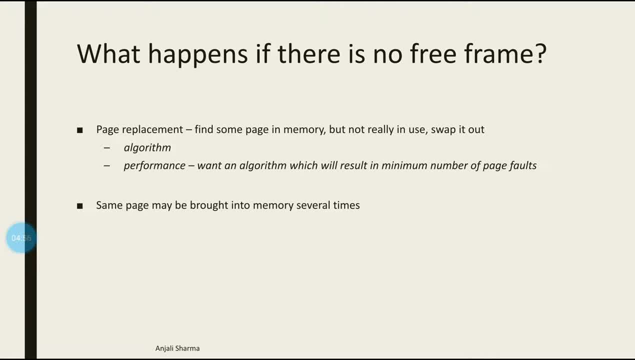 In the illustration of demand, paging and animation. we had seen that the page which is in the physical memory for a long time, which is the most longer waited page in the memory, we had removed it. So, basically, to replace the page, there must be a criteria for replacement right. 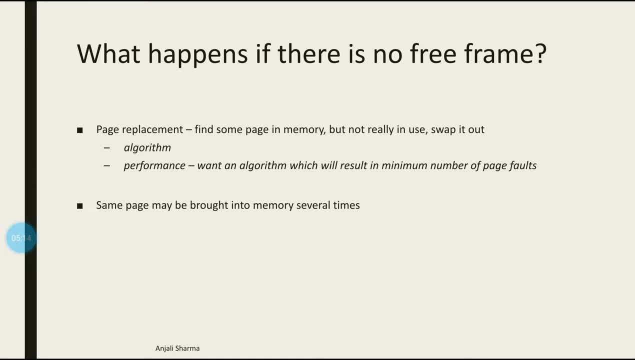 So that criteria is the algorithm. So what? basically, page replacement is finding a page from the memory which is not really in use and that's swapping it out from the memory, And for that we require an algorithm. that is the criteria And the basic thing of that algorithm is its performance, that we want our algorithms as such. 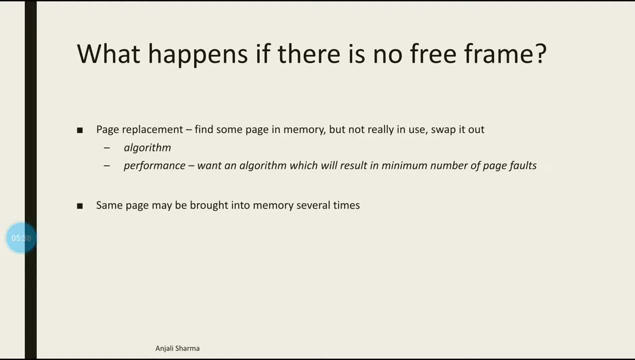 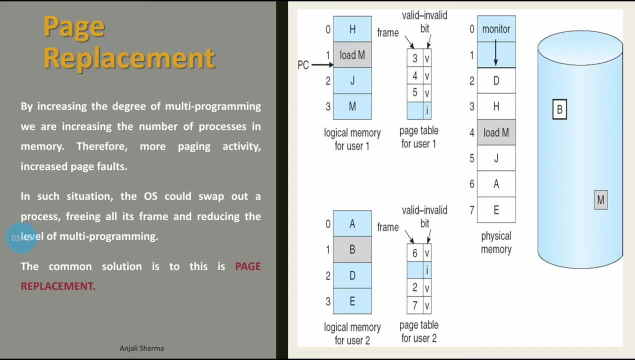 which will result in minimum number of page fault, An algorithm which has minimum number of page fault, because page fault is an overhead for us. So let us now see more technically, what is page replacement? It says that It says that by increasing the degree of multi-programming, 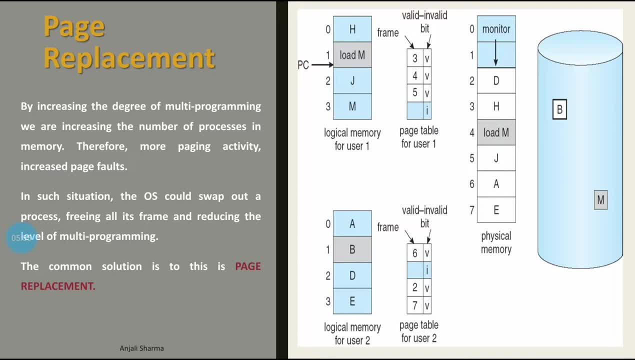 we are increasing the number of processes in the memory. Therefore more paging activity and increased page fault. See: the degree of multi-programming is at a point of time. how many programs are there in our main memory right? So if we increase the degree of multi-programming, then more programs will be in the memory. 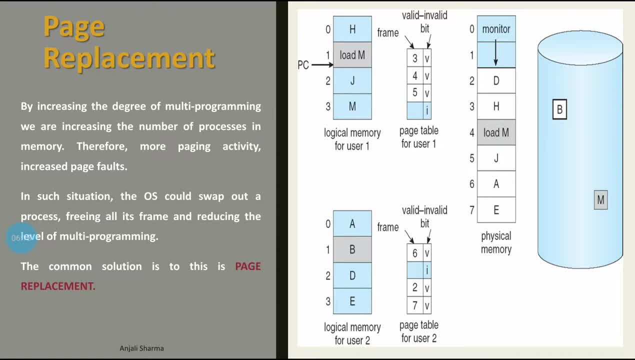 That means more pages will be in the memory. So if we try to refer more pages then the memory will be filled up. because we have increased the degree of multi-programming So we will have to perform page replacement again and again. So basically the degree of multi-programming is directly proportional to the frequency of page replacement. 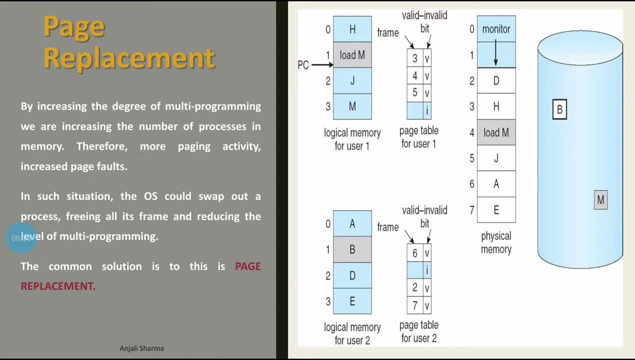 So in that scenario, what operating system deliberately does is just decrease the level of multi-programming, And that is written here. In such situation, the OS could swap out a process, freezing all its frames and thus reducing the level of multi-programming. 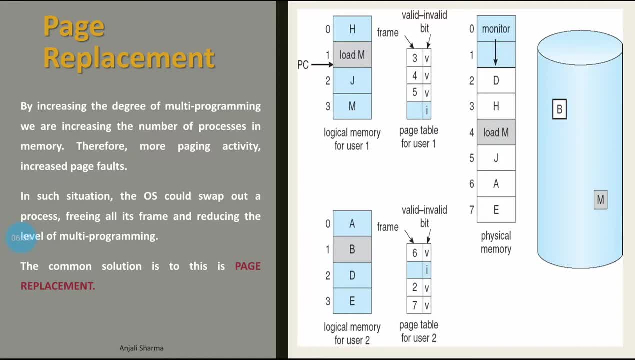 And this is done by the page replacement. So in such a situation operating system reduces the degree of multi-programming a little bit So that we can get some free frames and we can occupy the rest of the processes in the memory. So the concept of swapping and swap out can be reduced a little bit. 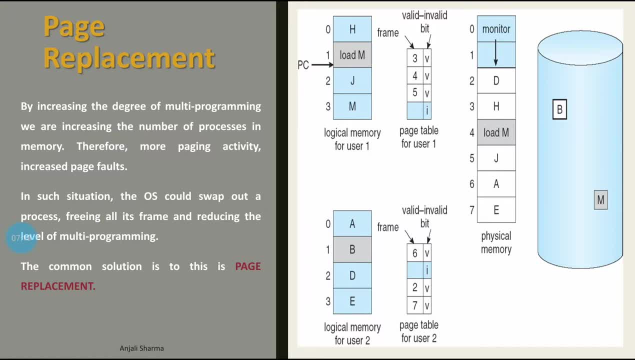 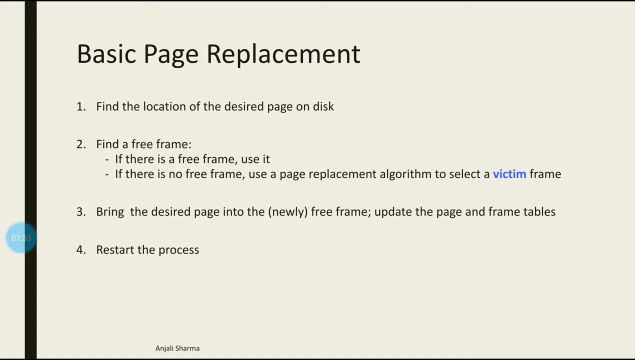 So that the frequency of page fault can be reduced a little bit. So that is page replacement, And we also have its algorithms, which we will discuss in the next video. So let's see the basic procedure of page replacement. It says that first go and find out the location of the desired page on the disk. 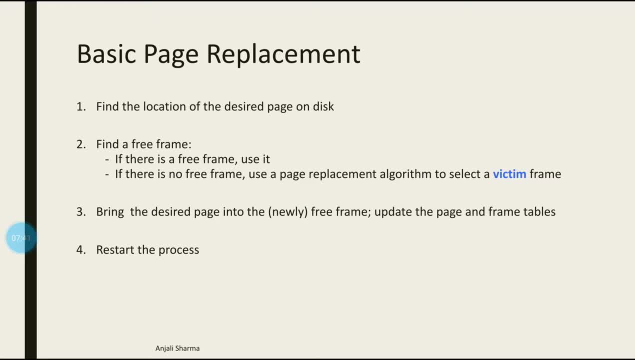 So first of all, the one who has to be swapped in the disk, That is, we identify the location in the hard disk, Then find a free frame. Then what is done? A free frame is identified in the memory. If we find a free frame, then put that missing page in that frame. 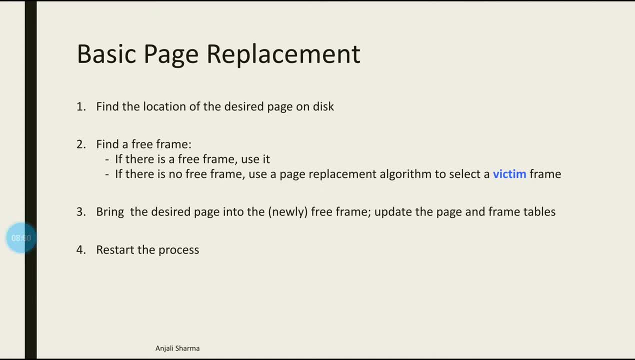 Suppose, if we do not find any free frame, then use a page replacement algorithm to select a victim frame. That means if the memory is full and we do not have any empty frame, then a frame will be selected Because if we remove the page from that frame and keep it in the backing store. 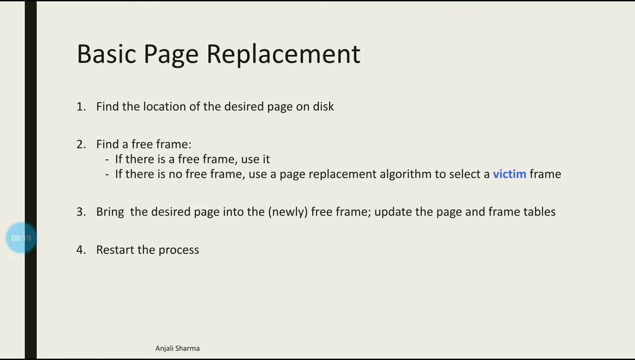 then it is given a terminology that it is a victim frame, Because we are taking the main memory from it and removing it from the main memory. So it is a victim frame And to select this we have different algorithms such as FIFO and optimal page replacement. 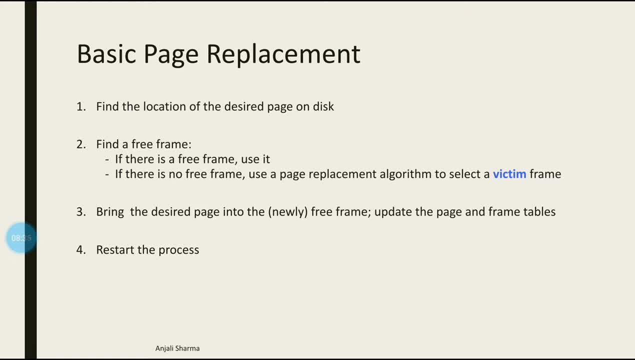 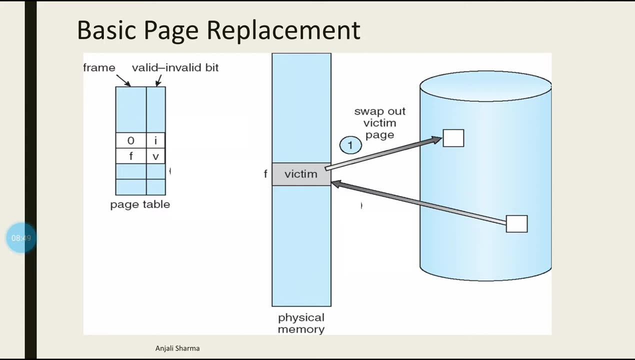 Bring the desired page into the free frame and update the page in the frame table And finally restart your process. So that was the page replacement. Let us see it diagrammatically. The first step will be finding out the victim process with the help of your algorithm. 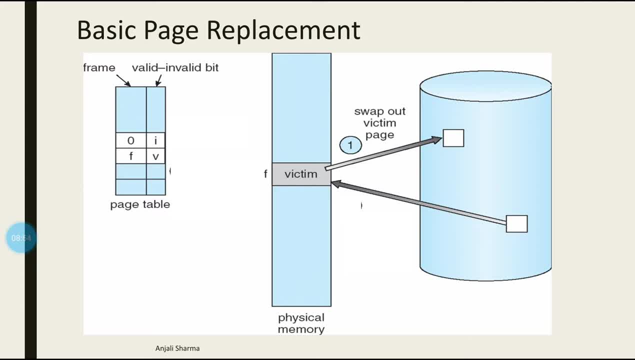 and swap out the victim page and put it back into the backing store. Accordingly, change the status of the valid and invalid bit to invalid, because now the page is no longer in the physical memory. The third step is swapping the desired page In the free frame. 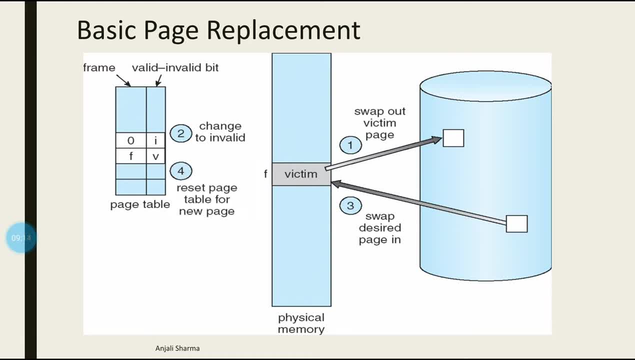 swap in the desired page and then again reset the page table for the new page, Because now the status of that particular page will be valid, because now it belongs to the physical memory. So that was the basic page replacement procedure. The last topic in this video will be the concept of modify bit. 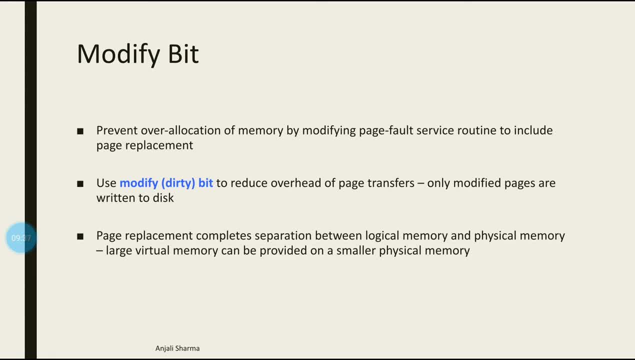 It says that prevent the over allocation of memory by modifying the page fault service routine to include page replacement. Use a modify, also known as a dirty bit, to reduce overhead of the page transfers and modify page table. Pages are only written to the disk. Page replacement completes separation between logical memory and physical memory. 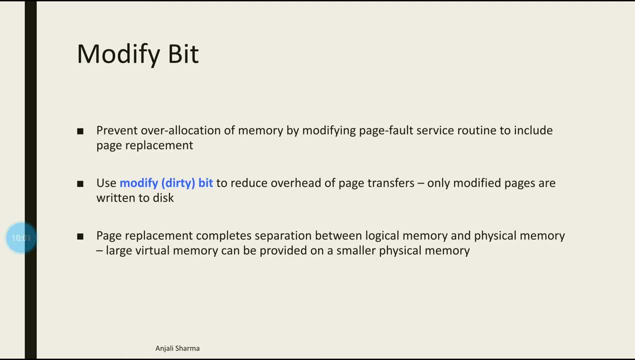 Large virtual memory can be provided on a smaller physical memory, So it seems a little overwhelming to listen to. I don't understand it at all, But it's a very easy concept, Just like we have associated a valid-invalid bit or read-only bit with a page. 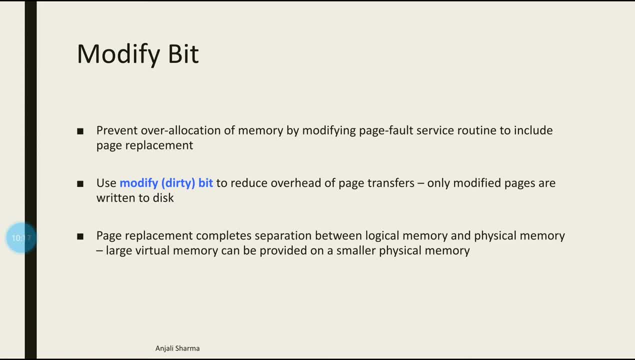 we also associate a modify bit in the same way. Modify bit means that recently, if the modify bit is set to 1, that means some modification has been done in the page, And it is assumed that if a page is recently visited, we might be able to visit it in the near future. 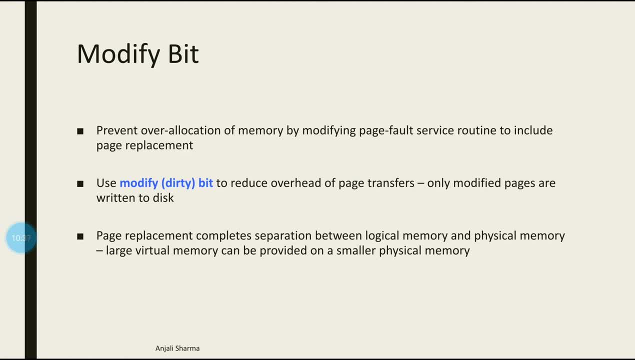 Because it is modified now it might be referred again. So in that scenario we don't replace that page and give it a chance. So that is a modify bit, And if that modify bit is 0, that means we haven't referred that page yet. 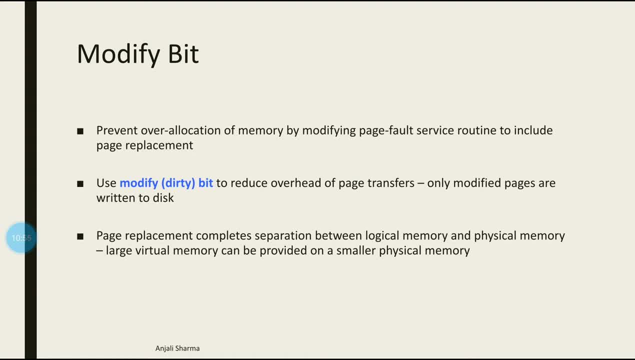 So when it's been a long time and we haven't referred that page in memory, then the chances of referring it in the near future will be very low. So what can we do? through a modify bit here We can identify the victim frame. 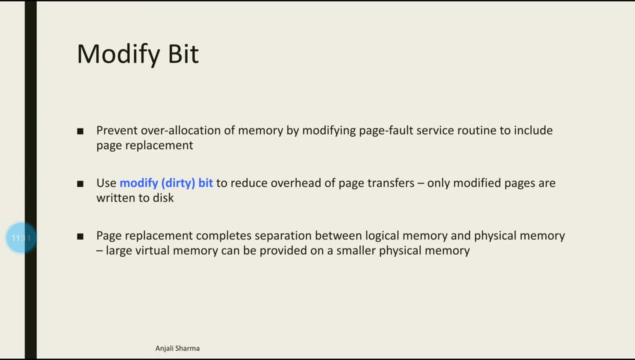 So basically what we did: we are just adding an additional bit, that is the modify bit, with our pages, And if it is set to 1, that means the page has been modified recently, So there is a more chance that it will be referred in the future.